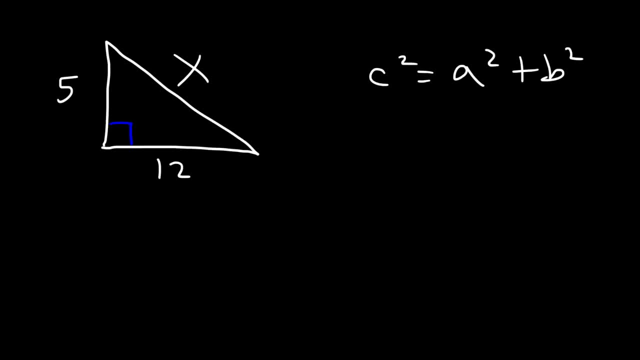 equal to A squared plus B squared. So A can be 5 or 12, it doesn't matter. So let's say if we choose A to be 12 and B is 5.. The hypotenuse C is across the box, which is X. So we have X squared is equal to 12. 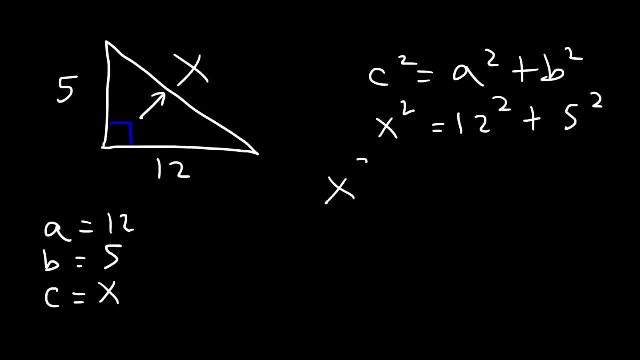 squared plus 5, squared Now 12 times 12 is 144 and 5 squared is 25.. 144 plus 25 is 169.. Now, to calculate the value of X, we need to take the square root of both sides. The square root of 169 is 13, and so that's how you can calculate the. 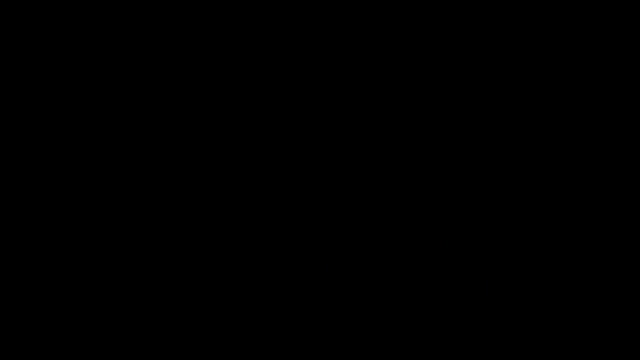 hypotenuse of a right triangle. Now let's work on another example. So let's say the hypotenuse is 10,, this is 5, and our goal is to calculate Y. Go ahead and do this, So let's use the same formula: C squared is equal to A squared. 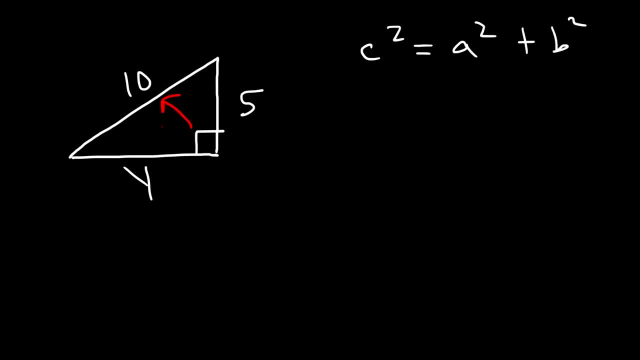 plus B squared. So C is the hypotenuse. So in this problem C is 10.. A, we could say it's Y, and then B is 5.. So it's going to be: 10 squared is equal to Y squared plus 5. squared 10 times 10 is 100 and 5 squared is 25.. 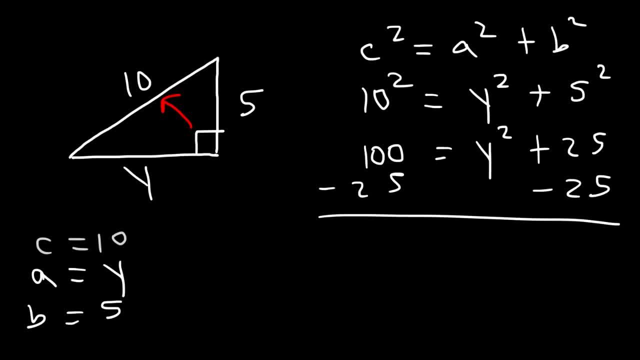 So we need to subtract both sides by 25.. Now 100 minus 25 is 75.. So now our next step is to take the square root of both sides, So Y is equal to the square root of 75.. Now how can we simplify this value to get the right answer or to get the exact answer in? 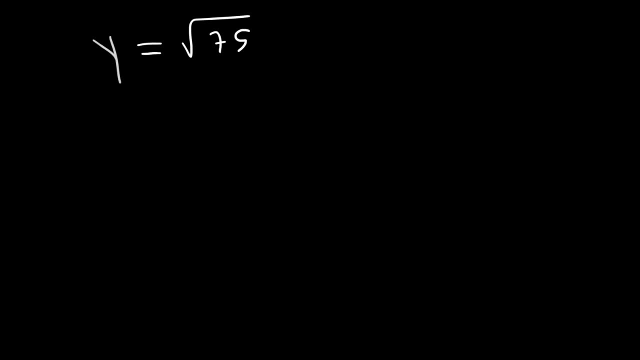 its fully simplified form. What perfect square goes into 75?? 25 is a perfect square that goes into it. 25 times 3 is 75 and the square root of 25 is 5.. So Y is equal to 5 square root 3.. 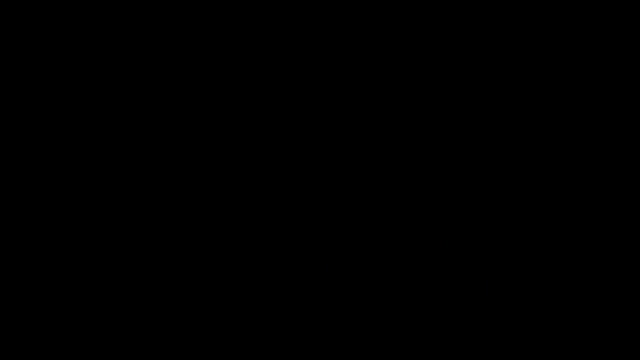 hypotenuse of a right triangle. Now let's work on another example. So let's say the hypotenuse is 10,, this is 5, and our goal is to calculate Y. Go ahead and do this, So let's use the same formula: C squared is equal to A squared. 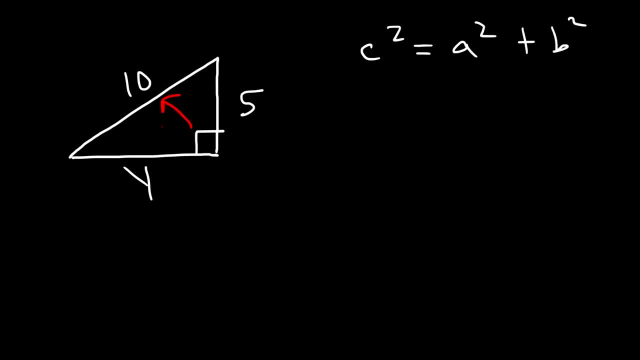 plus B squared. So C is the hypotenuse. So in this problem C is 10.. A, we could say it's Y, and then B is 5.. So it's going to be: 10 squared is equal to Y squared plus 5. squared 10 times 10 is 100 and 5 squared is 25.. 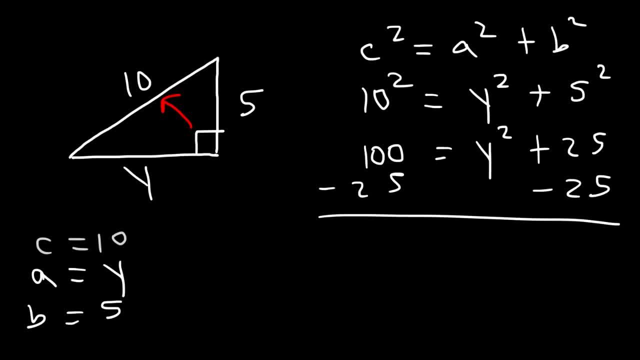 So we need to subtract both sides by 25.. Now 100 minus 25 is 75.. So now our next step is to take the square root of both sides, So Y is equal to the square root of 75.. Now how can we simplify this value to get the right answer or to get the exact answer in? 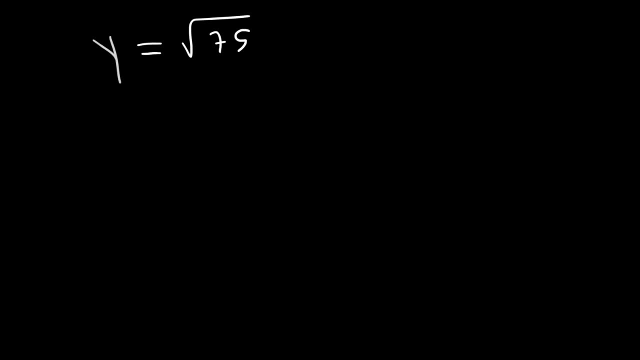 its fully simplified form. What perfect square goes into 75?? 25 is a perfect square that goes into it. 25 times 3 is 75 and the square root of 25 is 5.. So Y is equal to 5 square root 3.. 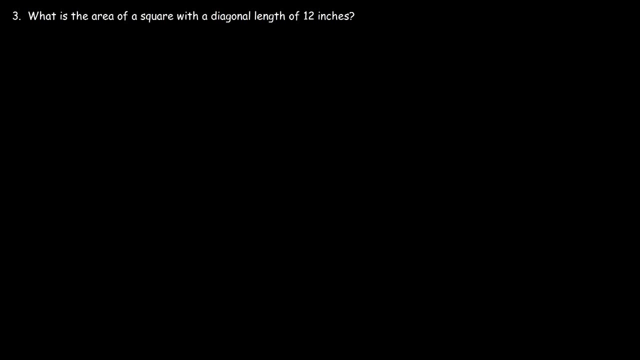 Now let's work on some word problems. What is the area of a square with a diagonal length of 12 inches? So first let's draw a square, And so this is just a rough sketch of a square, And this is the diagonal of the. 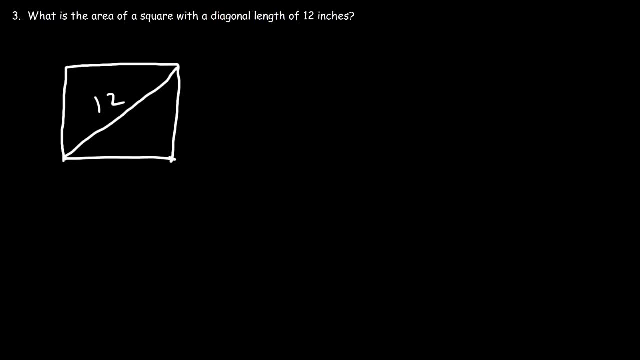 square, So that's 12.. Now let's call this X. All four sides of a square are the same, so this is X. So notice that we have a right triangle. The area of a square is the length times the width. Both the length and the width is equal to X, So 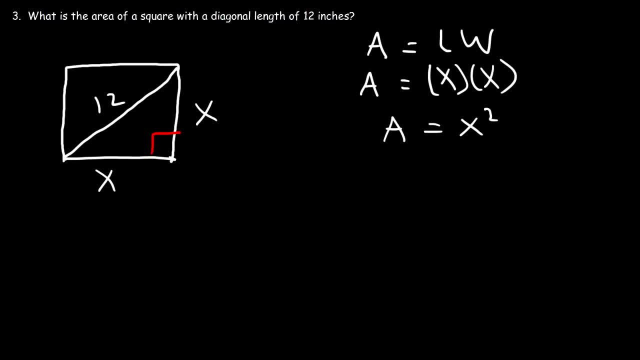 the area of a square is X squared. So if we can calculate the value of X, we can calculate the area of the square. So let's use the Pythagorean theorem to calculate X. So C squared is equal to A squared plus B squared C, the hypotenuse is 12.. A is equal to X in this example. 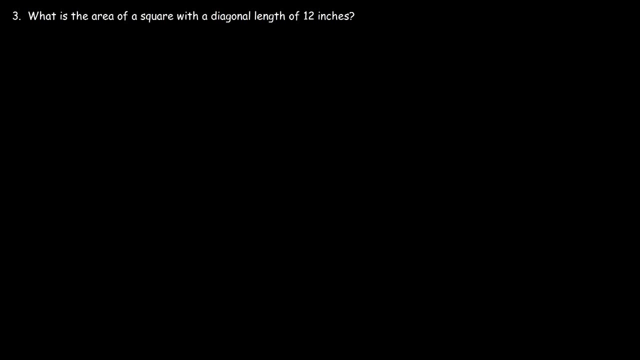 Now let's work on some word problems. What is the area of a square with a diagonal length of 12 inches? So first let's draw a square, And so this is just a rough sketch of a square, And this is the diagonal of the. 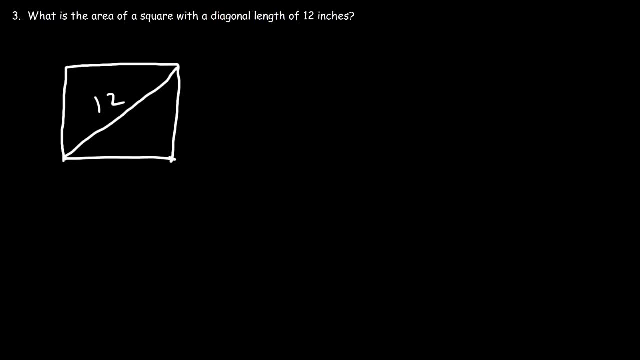 square, So that's 12.. Now let's call this X. All four sides of a square are the same, so this is X. So notice that we have a right triangle. The area of a square is the length times the width. Both the length and the width is equal to X, So 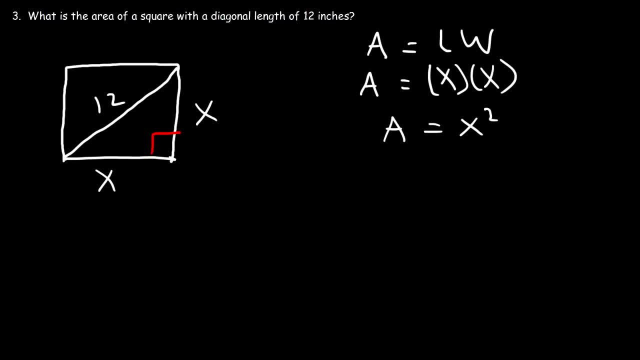 the area of a square is X squared. So if we can calculate the value of X, we can calculate the area of the square. So let's use the Pythagorean theorem to calculate X. So C squared is equal to A squared plus B squared C, the hypotenuse is 12.. A is equal to X in this example. 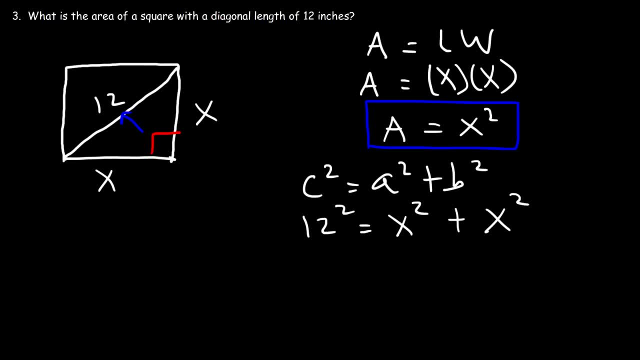 and B is equal to X. So 12 squared is X squared plus X squared, 1x squared plus 1x squared is 2x squared And 12 squared is 144.. So first we need to divide both sides by 2.. 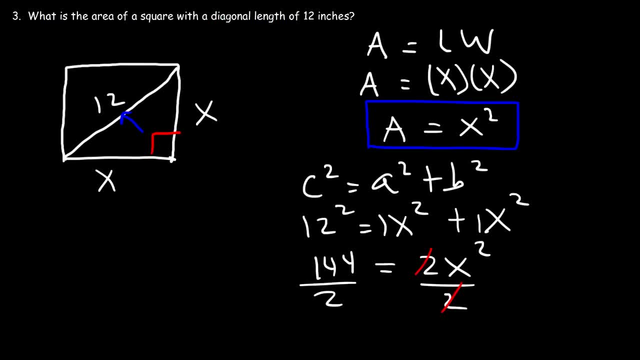 144 divided by 2 is 72. And so that's equal to X squared. Now let's take the square root of both sides. So X is equal to the square root of 72.. Now A is equal to X squared, And X squared is 72. So A is just 72.. So that's the area of the square. 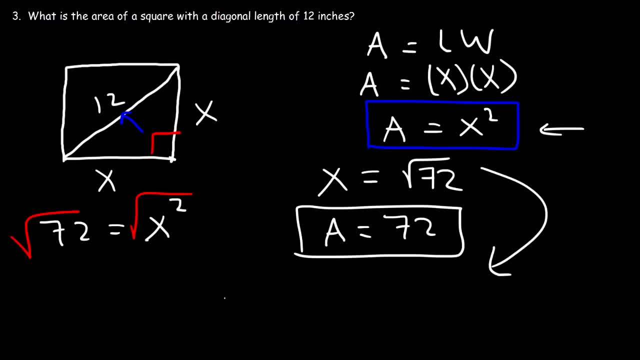 By the way, if you want to simplify this radical, you can say that 72 is 36 times 2. And the square root of 36 is 6.. So X is 6 square root 2. But the area is X squared. 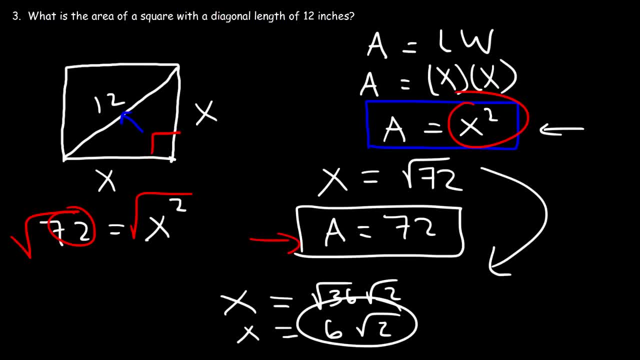 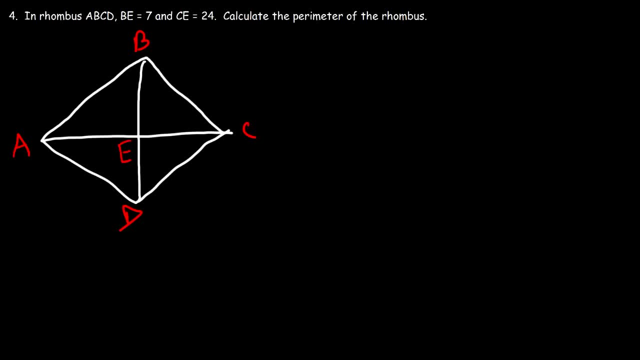 And we can see that X squared is 72, which means A is 72 in this example, Number 4.. In rhombus, A, B, C, D, B, E is 7 and C, E is 24.. 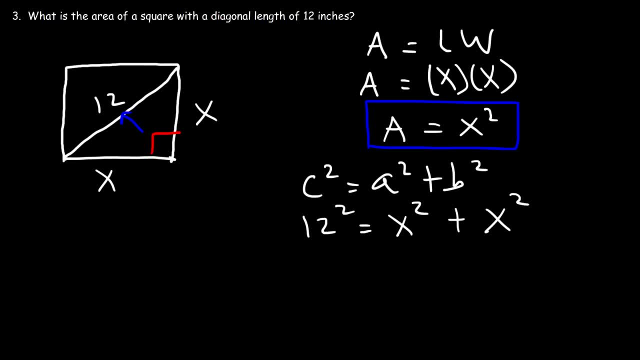 and B is equal to X. So 12 squared is X squared plus X squared, 1x squared plus 1x squared is 2x squared And 12 squared is 144.. So first we need to divide both sides by 2.. 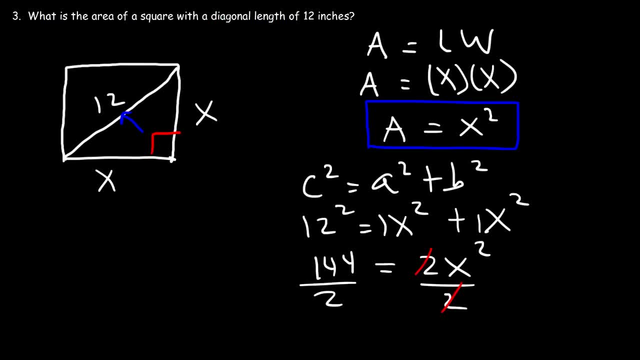 144 divided by 2 is 72. And so that's equal to X squared. Now let's take the square root of both sides. So X is equal to the square root of 72.. Now A is equal to X squared, And X squared is 72. So A is just 72.. So that's the area of the square. 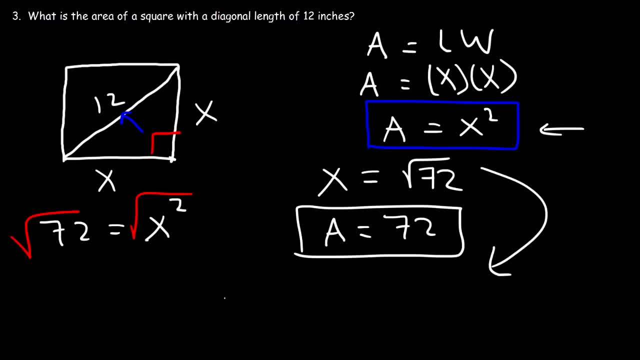 By the way, if you want to simplify this radical, you can say that 72 is 36 times 2. And the square root of 36 is 6.. So X is 6 square root 2. But the area is X squared. 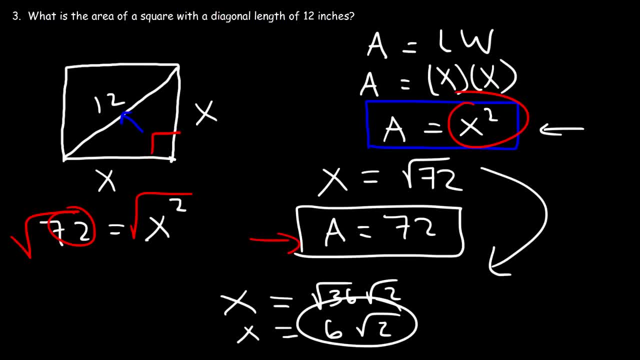 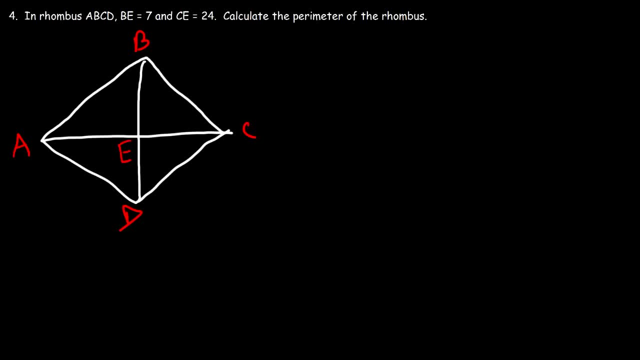 And we can see that X squared is 72, which means A is 72 in this example, Number 4.. In rhombus, A, B, C, D, B, E is 7 and C, E is 24.. 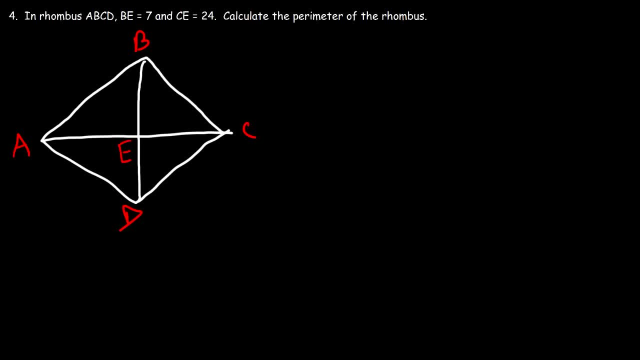 Calculate the perimeter of the rhombus. So the first thing you need to know is that the diagonals of a rhombus bisect each other at 90 degrees. B? E is 7 and C? E is 24.. Because of rhombus, the 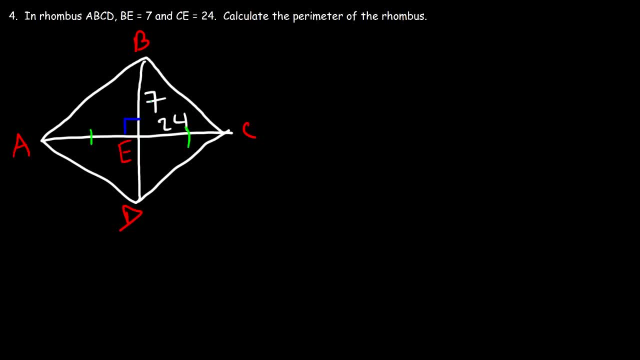 diagonals of a rhombus bisect each other. A, E and E C are congruent. B, E and E D are congruent, So if B, E is 7, E, D is 7.. 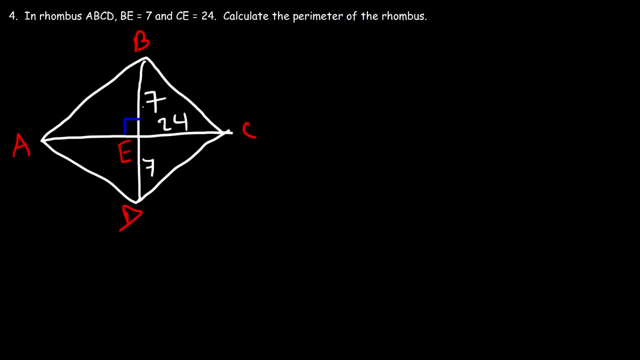 And if E- C is 24, A- E is 24.. Now, all four sides of a rhombus are congruent. So let's say: if we call this S, This is S, that's S, that's S. So the perimeter is 4S. 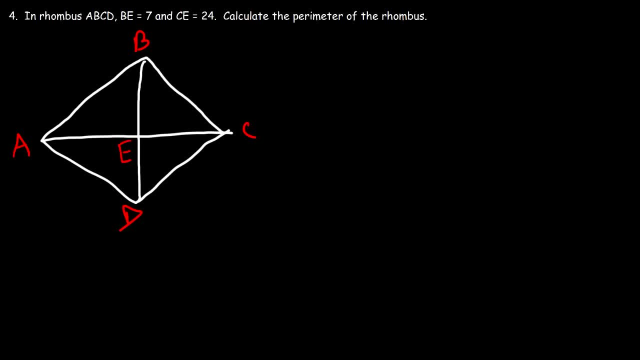 Calculate the perimeter of the rhombus. So the first thing you need to know is that the diagonals of a rhombus bisect each other at 90 degrees. B? E is 7 and C? E is 24.. Because of rhombus, the 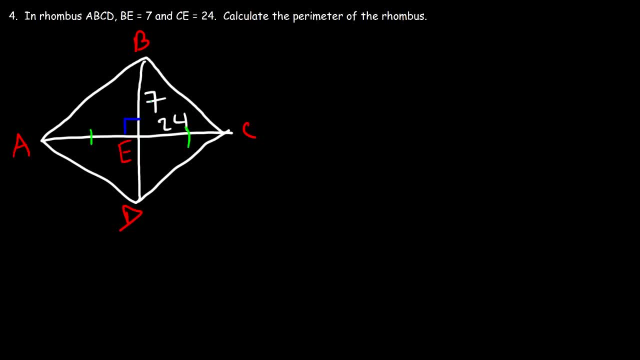 diagonals of a rhombus bisect each other. A, E and E C are congruent. B, E and E D are congruent, So if B, E is 7, E, D is 7.. 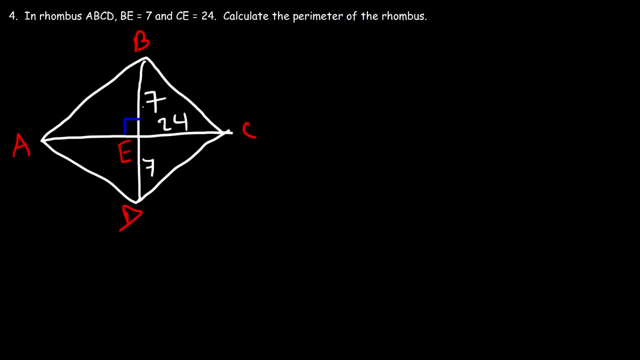 And if E- C is 24, A- E is 24.. Now, all four sides of a rhombus are congruent. So let's say: if we call this S, This is S, that's S, that's S. So the perimeter is 4S. 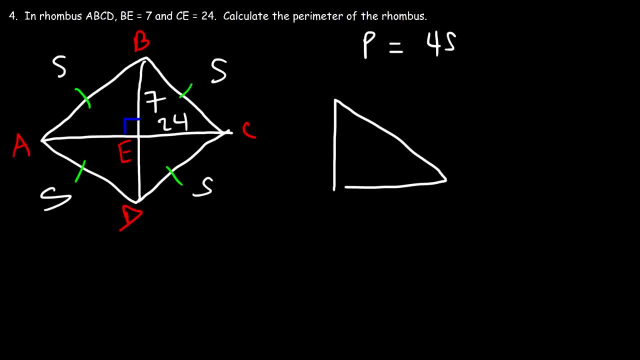 Now notice that we have 4S, But we also have 4 congruent right triangles. This is 7,, this is 24, and this is S. So let's use the Pythagorean theorem to calculate S. C squared is equal to A squared plus B squared. In this case, C is the hypotenuse S. 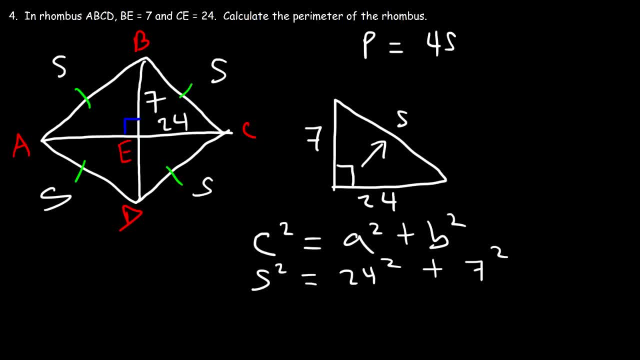 A, we could say, is 24, and B is 7.. 24 times 24.. that's 576.. 7 squared is 49. now 576 plus 49 is 625. so now let's take the square root of both sides. the square root of 625 is 25, so now we can calculate the perimeter. so 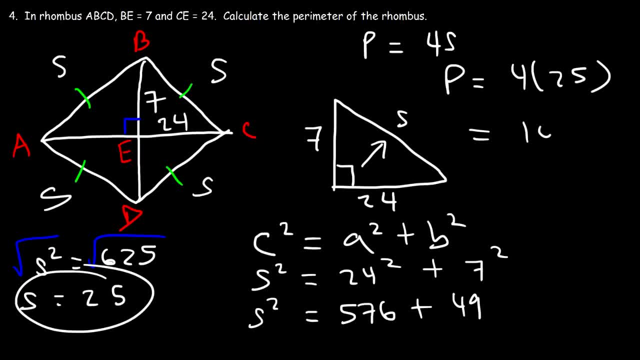 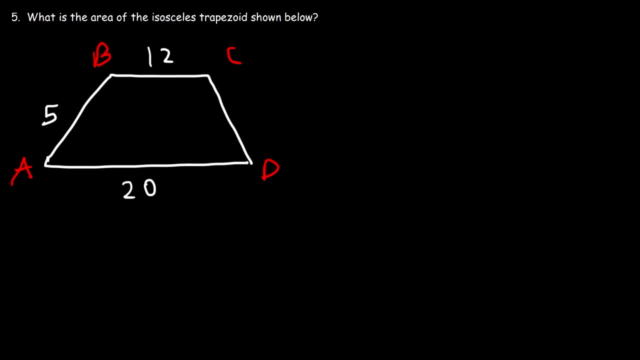 it's 4s, or 4 times 25, which is a hundred. so that's the perimeter for this particular rhombus. it's a hundred units number five: what is the area of the isosceles trapezoid shown below? so first we need the formula. the area is one. 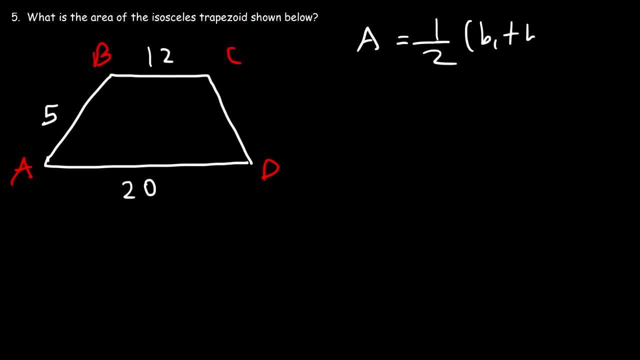 half b1 plus b2 times H. so b1 is the first base and b2 is the first base and b1 is the first base and b1 is the first base, and that's 12. b2 is the second base, which is 20, and H is the height of the. 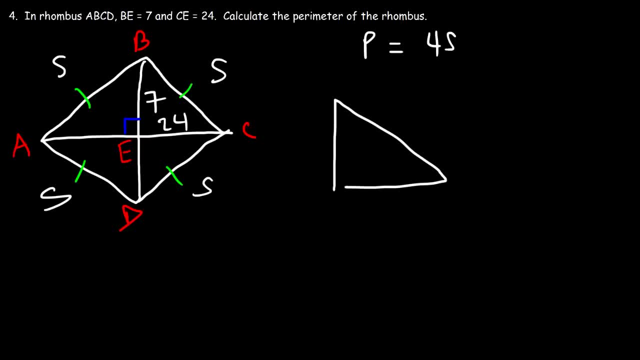 Now notice that we have 4S. We have 4 congruent right triangles. This is 7,, this is 24, and this is S. So let's use the Pythagorean Theorem to calculate S. C squared is equal to A squared plus B squared. In this case, C is the hypotenuse S. 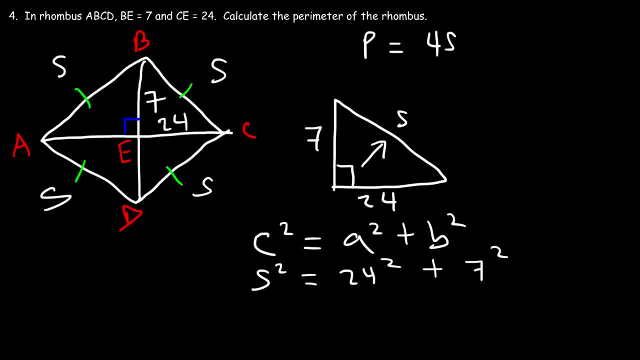 A, we can say it's 24, and B is 7.. 24 x 24, that's 576.. And 7 squared is 49.. Now 576 plus 49 is 625.. So now let's take the square root of both sides. 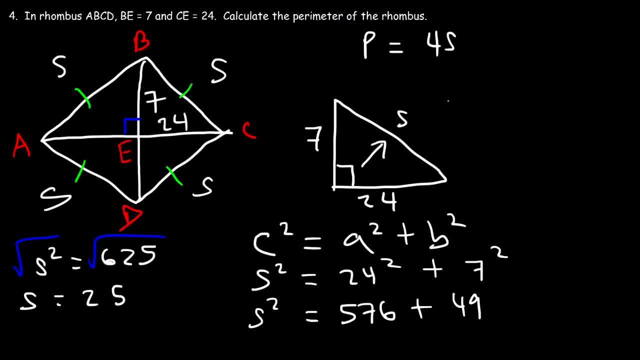 The square root of 625 is 25.. So now we can calculate the perimeter. So it's 4s, or 4 times 25, which is 100.. So that's the perimeter for this particular rhombus: It's 100 units. 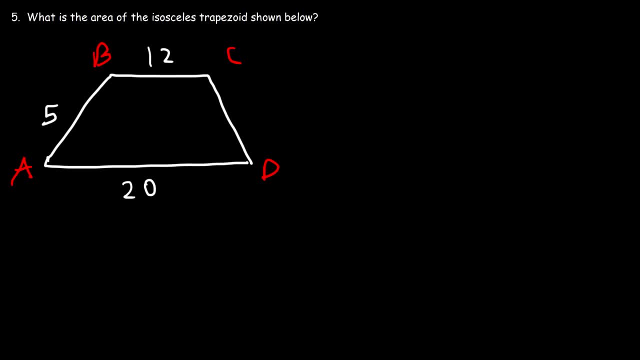 Number 5.. What is the area of the isosceles trapezoid shown below? So first we need the formula. The area is 1 half b1 plus b2 times h, So b1 is the first base, that's 12.. 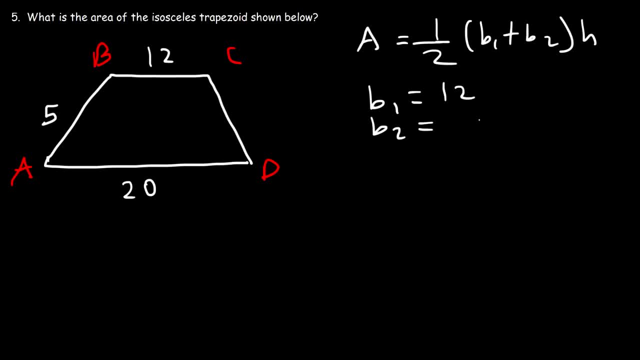 b2 is the second base, which is 20.. And h is the height of the trapezoid. So somehow we'll need to calculate h in order to calculate the area. So how can we do so? Now, the first thing we need to realize is that for an isosceles trapezoid, ab is congruent. 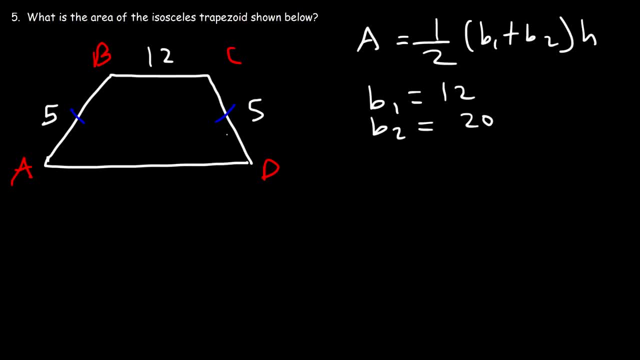 to cd. So both sides are equal to 5.. So that's the area. Next we need to draw two right triangles. Now we know that ad is 20.. That was given to us in the beginning. Now, if we add two additional points, let's call this e and f. ef is the same as bc. 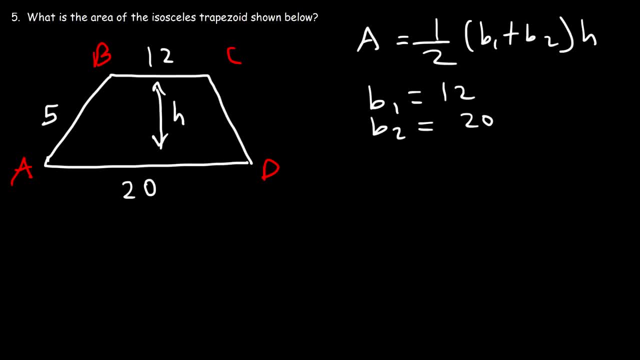 trapezoid. so somehow we need to calculate H in order to calculate the area. so how can we do so? now, the first thing we need to realize is that for an isosceles trapezoid, AB is congruent to CD, so both sides are equal to 5. next we need to 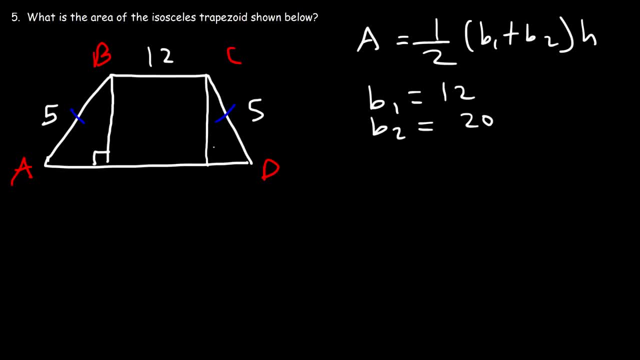 draw two right triangles. now we know that AD is 20. that was given to us in the beginning. now, if we add two additional points, let's call this E and F- E. F is the same as BC, that's 12. now if these two sides are congruent, 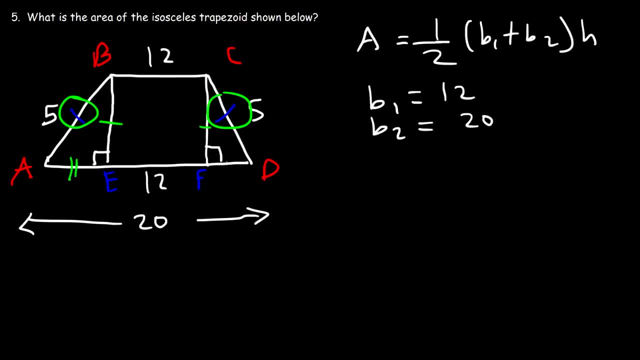 and this and that has to be congruent. these two, AD and FD, must be congruent to each other. so if we call this x and x, we could say that x plus 12 plus x is equal to 20, or 2 X plus 12 is equal to 20. so let's subtract both sides by 12. so 20 minus 12 is 8, and if we divide by 2 we can see the difference between those. and if we divide by 2, we can see the difference between those three. we can. So 20 minus 12 is 8. And if we divide by 2, we can see the difference between the. 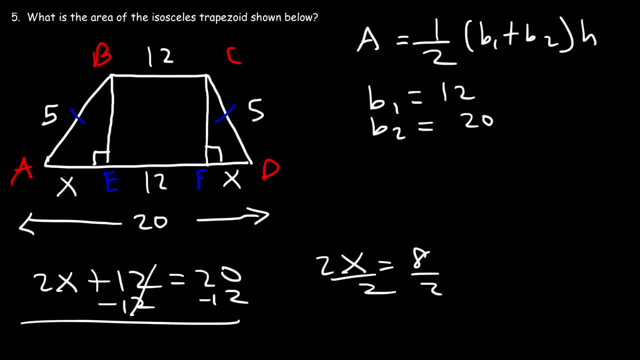 We can see that x is 4.. So we can put a 4 here. So now we can find h, the missing side. So now let's focus on this right triangle. c squared is equal to a squared plus b squared. The hypotenuse is 5.. 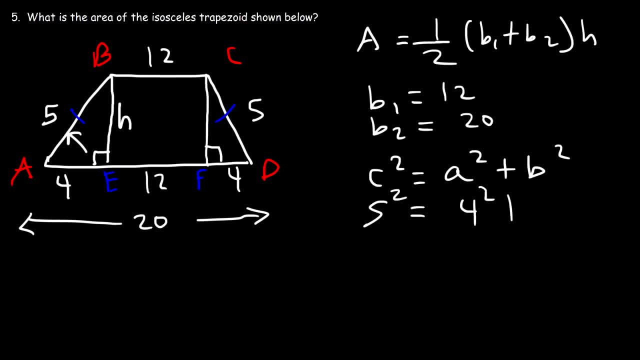 a we can say it's 4, and b is h. 5 squared is 25, 4 times 4 is 16.. And 25 minus 16 is 9.. So h squared is 9.. And if we take the square root of both sides we can see that h is equal to 3.. 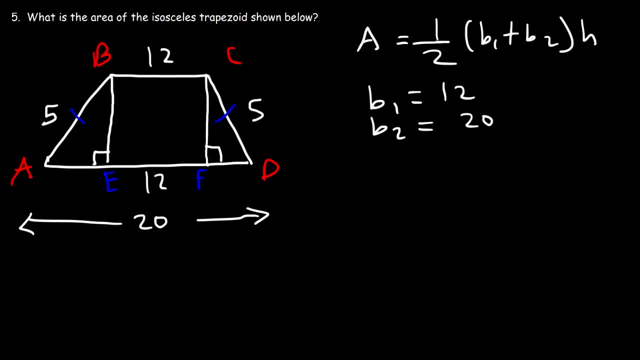 That's 12.. Now, if these two sides are congruent- and this and that have to be congruent- these two, ae and fd, must be congruent. They're congruent to each other. So if we call this x and x, we can say that x plus 12 plus x is equal to 20.. 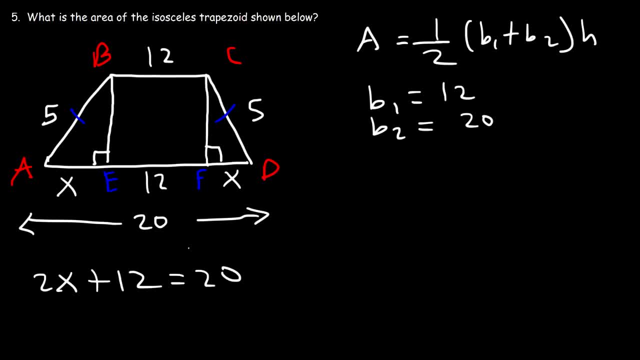 Or 2x plus 12 is equal to 20.. So let's subtract both sides by 12.. So 20 minus 12 is 8.. And if we divide by 2, we can see that x is 4.. Okay. 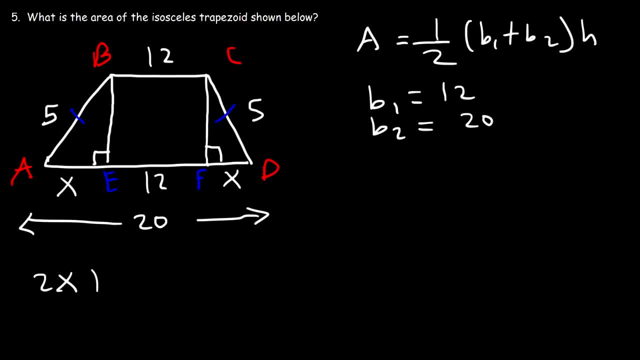 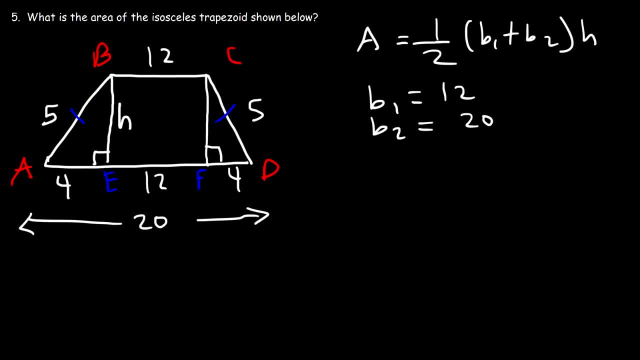 So now let's focus on this right triangle. C squared is equal to a squared plus b squared. The hypotenuse is 5.. A, we can say it's 4. And b is h. 5 squared is 25.. 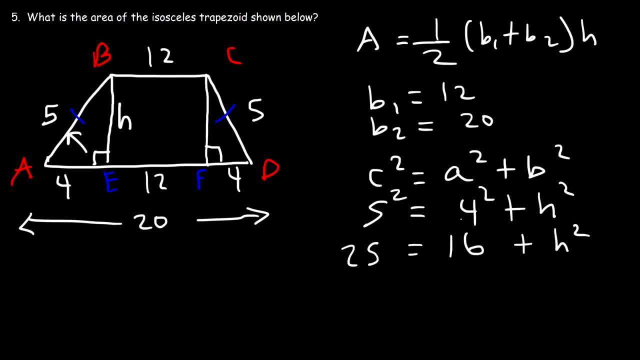 4 times 4 is 16.. and 25 minus 16 is 9. so H squared is 9 and if we take the square root of both sides we can see that H is equal to 3. so now that we have the value of H, we can. 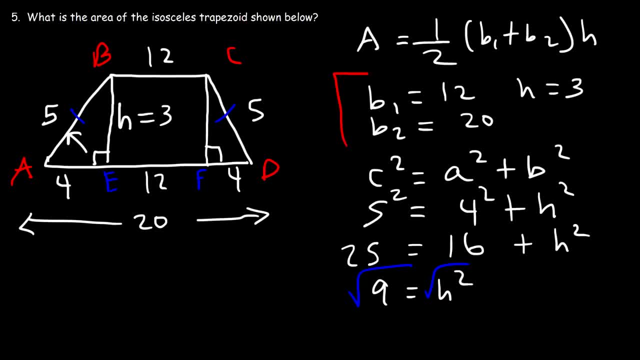 So now that we have the value of h, we can calculate the area of the trapezoid using this formula. That is this formula here. So it's going to be 1 half b1,, which is 12,, plus b2,, which is 20, times the height of 3.. 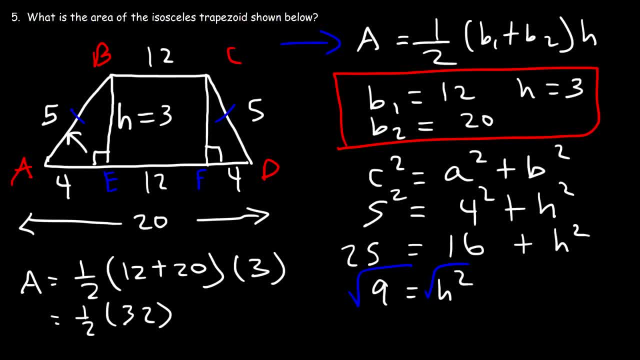 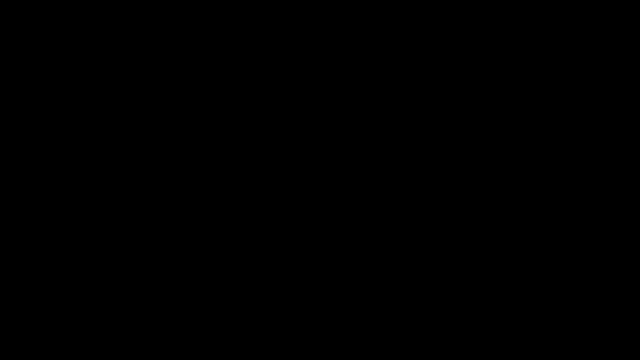 Now, 12 plus 20 is 32.. And half of 32 is 16.. 16 times 3 is 48.. So this right here is the answer. That's the area of the trapezoid. Answer isined to h's. 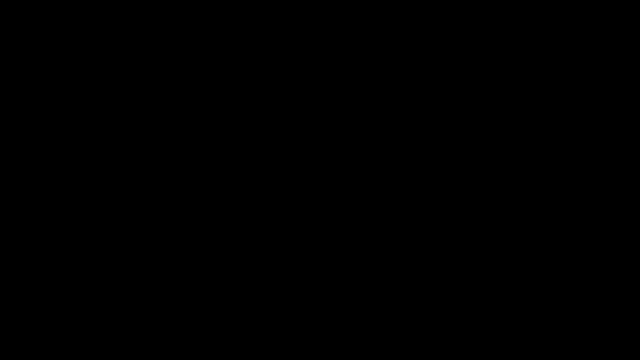 If you are asked in individual and claiming this, you can get each other h, which is 8.. 1 over 10.. fewer 16 plus b, equal to 3. 10 minus 6.. 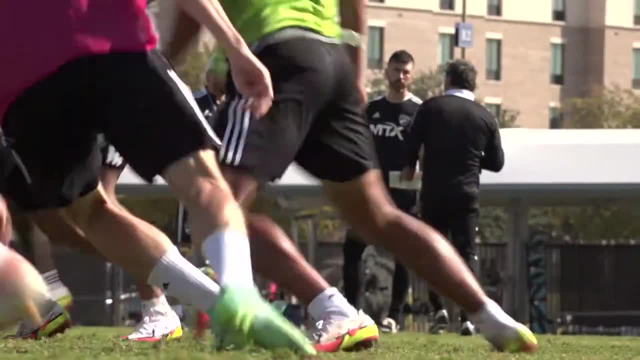 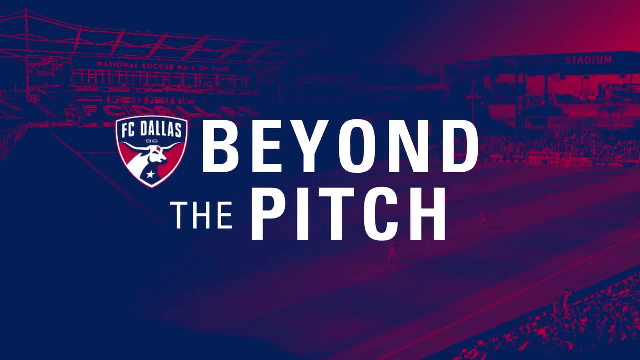 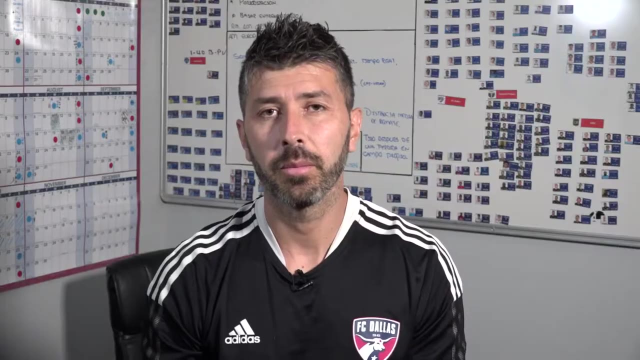 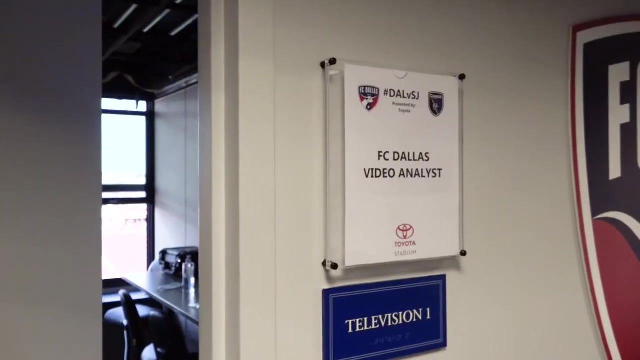 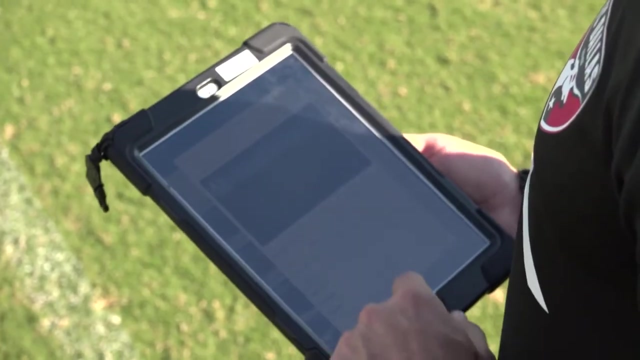 My name is Freddy Herrera and I'm the head of performance analysis at FC Dallas. Well, I've been with the club since 2017 and my main role here is opposition analysis. Through the week, we focus on our team training day to day, recording trainings, making sure 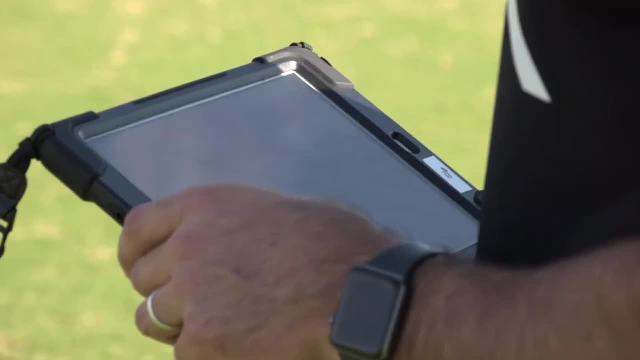 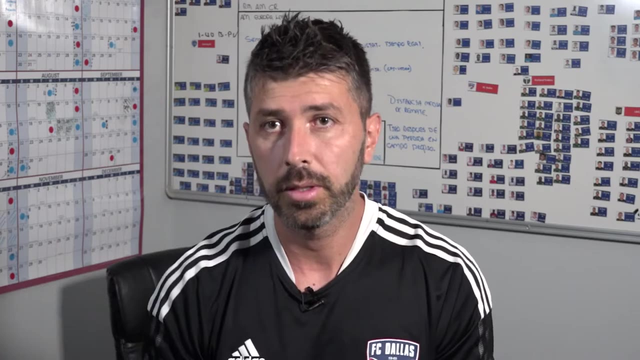 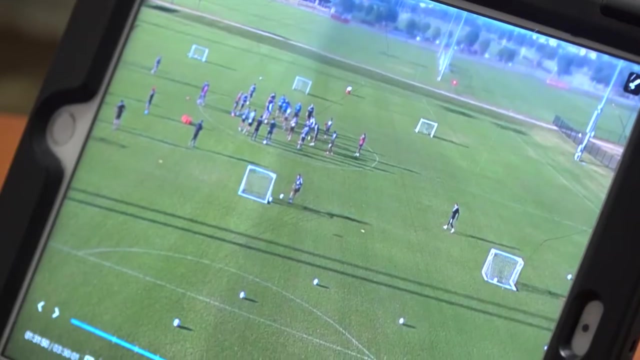 we share with the staff any analysis that we do. Even though we play and we're preparing for a game on the weekend, we are focusing, as an analysis, on the following game, so we're basically going a week ahead of the team in terms of analysis. 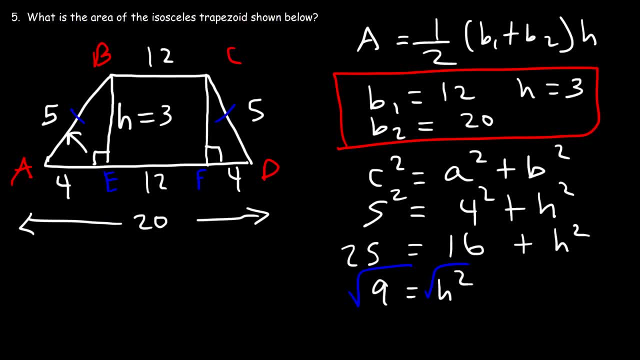 calculate the area of the trapezoid using this formula. that is this formula here. so it's going to be 1 half B 1, which is 12, plus B 2, which is 20 times the height of 3. now, 12 plus 20 is 32, and half of 32 is 16. 16 times 3 is 48. so 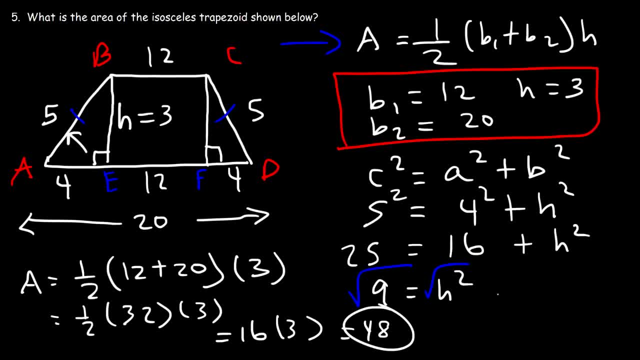 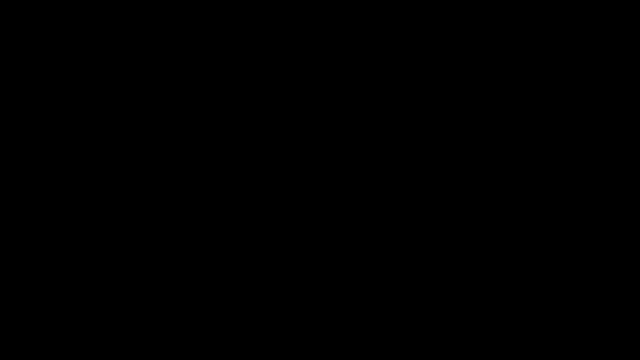 this right here is the answer. that's the area of the trapezoid, you.